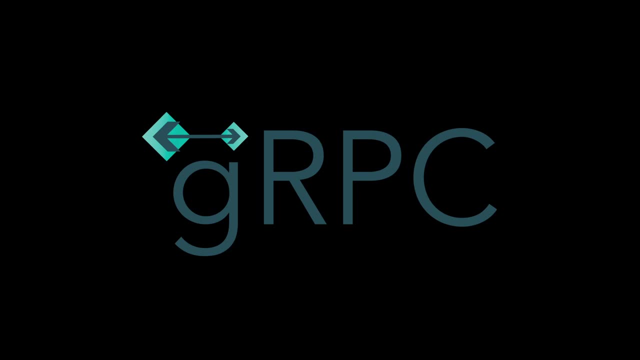 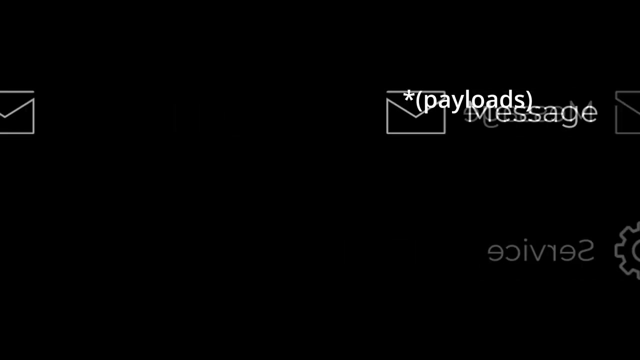 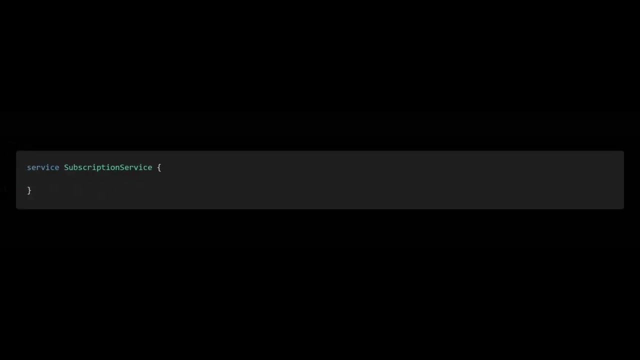 That's where JPEG is. The RPC comes in with two basic primitives: The protobuf message specifying your payloads And the service definition or your endpoints. Let's convert the payloads: first We create one protobuf for the request and one for the response. Then we create the service definition, containing one RPC. 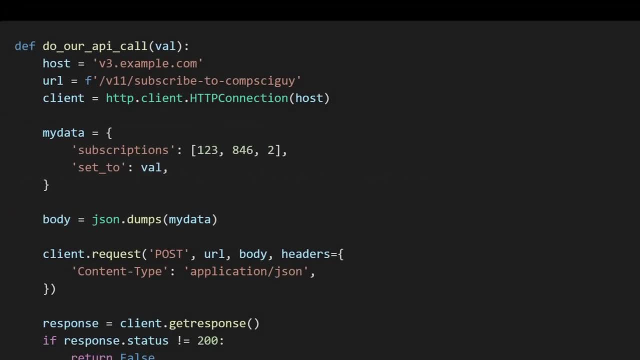 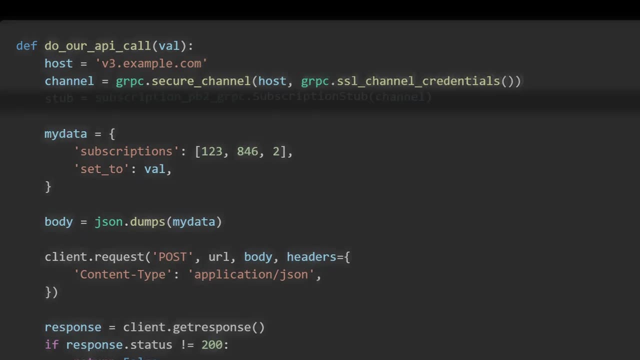 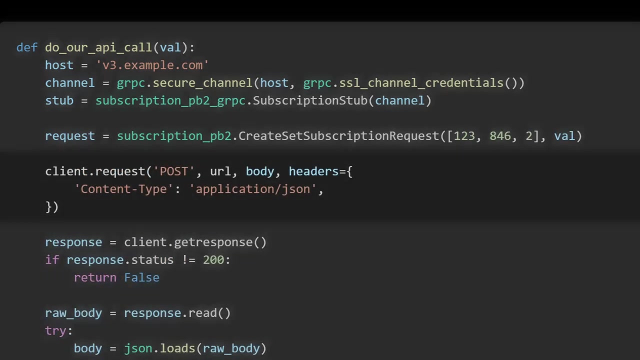 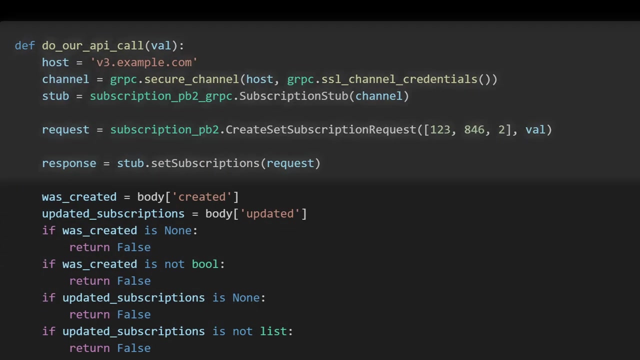 Set subscript. We use this by first switching the HTTP client with a gRPC channel, the server connection and a subscription service stub. We create the request, Pass it to the stub's set subscription method, which returns a response. Then we just use the response that was created and updated subscription. 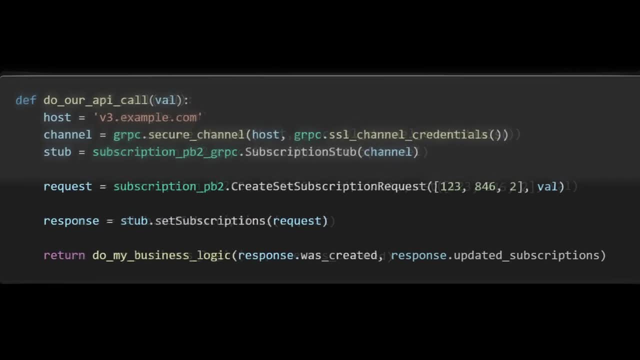 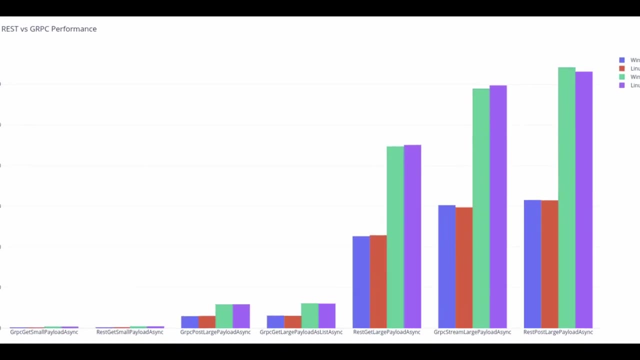 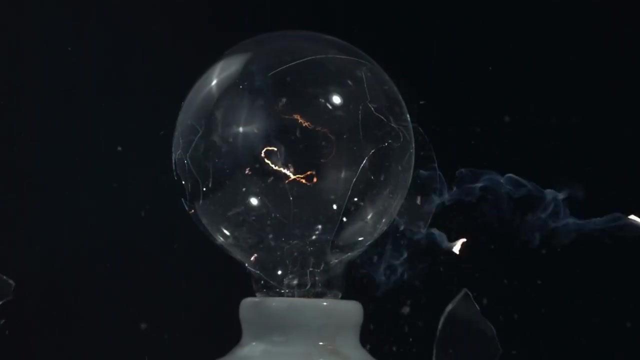 Then we just use the response that was created and updated subscription. If you contact the tool, we will let you know the response. Oh, and also, this is seven times faster than REST And you will never break your API, ever again. Now let's look at a larger example, Like this beautiful Python server. 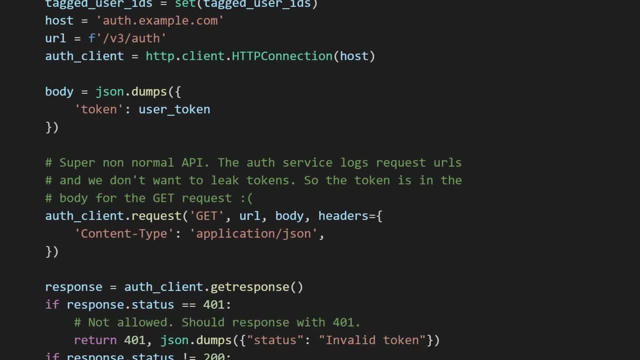 It is creating social media posts where we tag other users. We call an endpoint to authenticate a request. Then there is another endpoint. We call the request client and generate a request And we then set the protocol. We call it to keep Enable, as If it's using a你 beautifully- friendly request. There is a period for kannst tú 건�неать? Connor, who will declare a request, And the client becomes passive instead of individual users By white趨 É con quién, McCengerيف, we declare a request to this purpose. Then there is a check for Arthur Tarzans, who will run and ancestral. 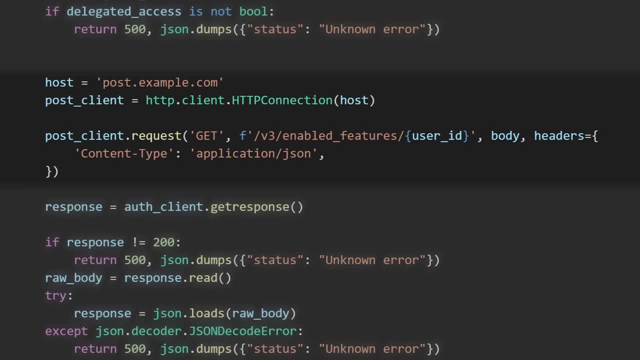 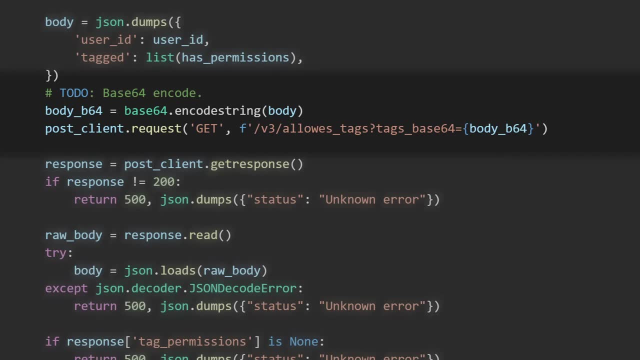 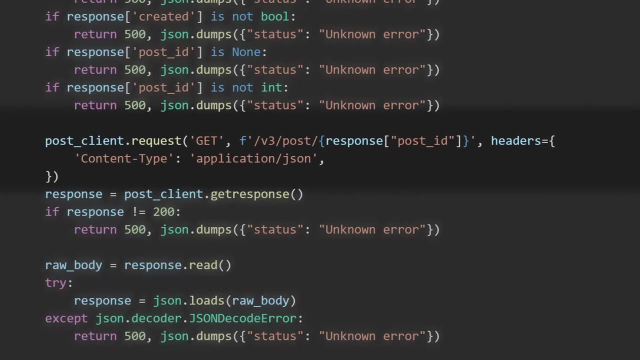 Then there is an endpoint to ensure the user is allowed to make posts for the account. We verify that the user may tag all the tagged users. Finally, we create the post and get it in the canonical format before returning the created post. So a lot of boilerplate. 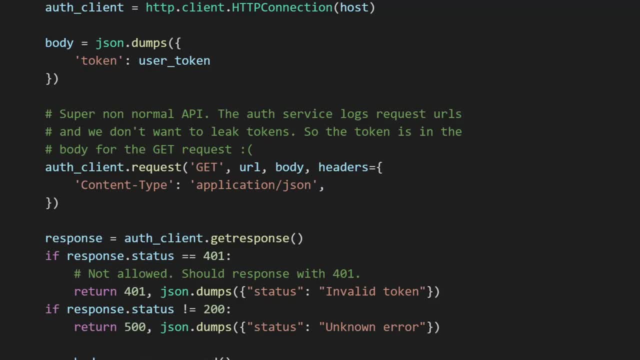 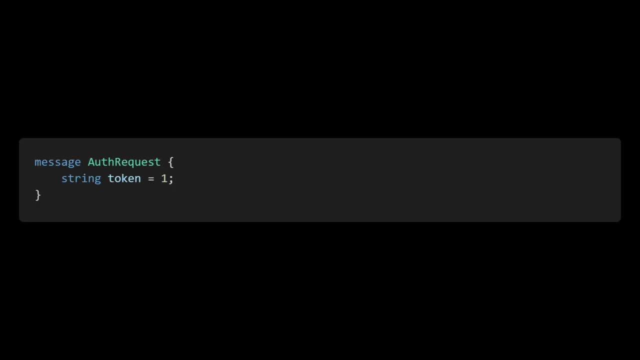 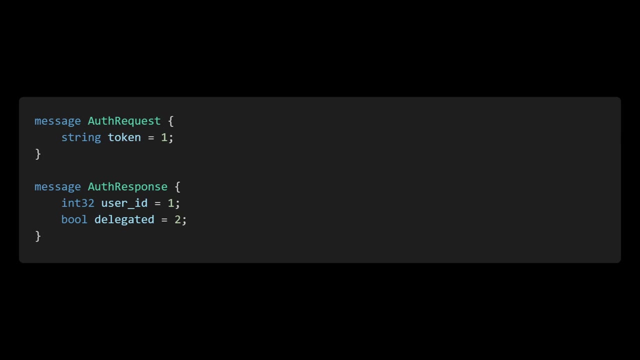 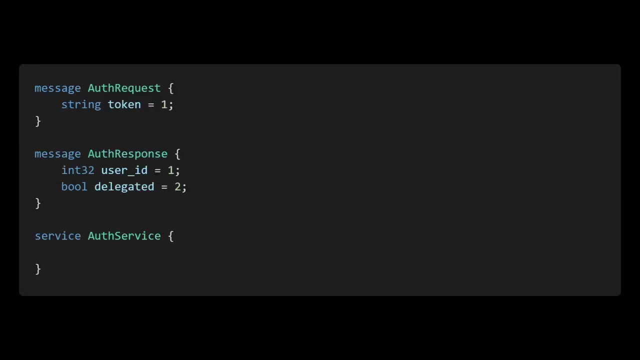 We start out with converting the off service from a REST API to a gRPC server. First create the request message, taking only the user's token, the response returning the user ID, and if it is delegated access, Then we create the service definition with just a single. 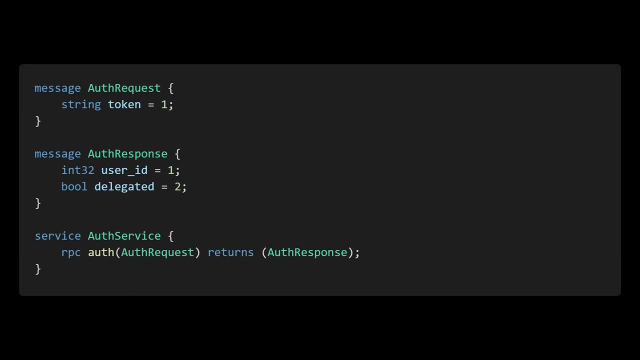 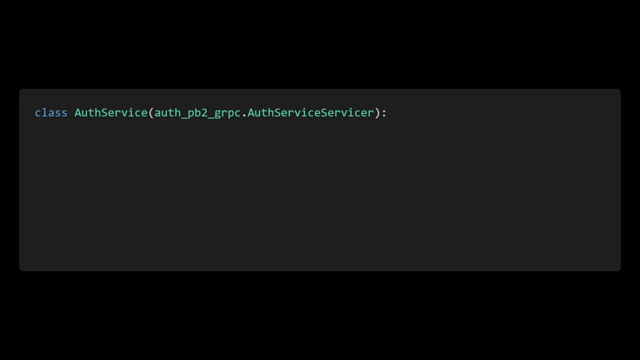 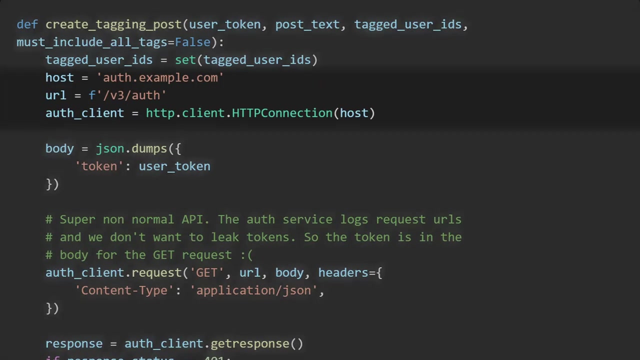 RPC off. To implement this, create a class off service inheriting the generated code off service services. Implement the off RPC returning permissions denied if the token is invalid. Now we just need to convert the client code as well. First, replace the HTTP client with the off service stub. 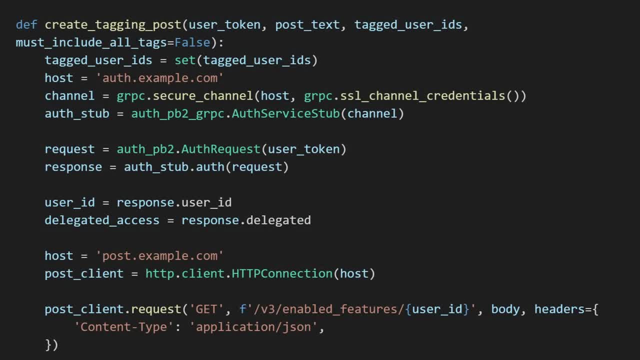 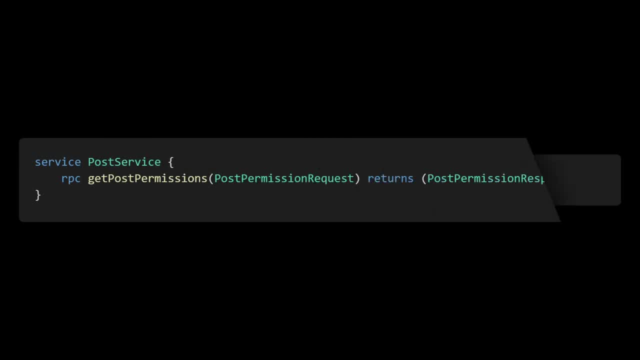 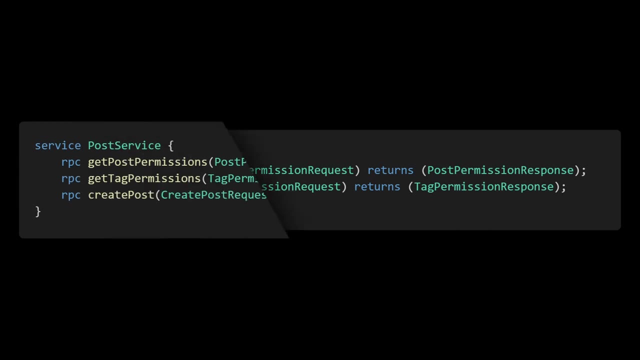 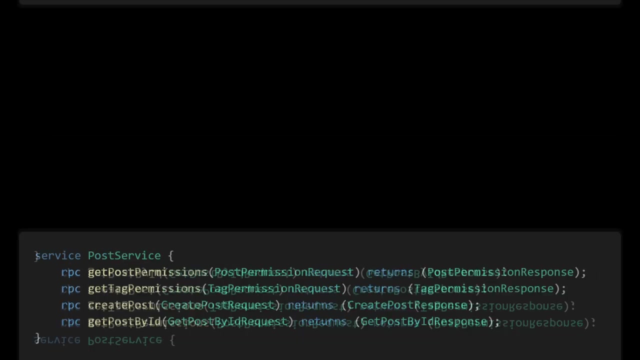 Send the off request and read the data from the response. Next we need to create the post service gRPC stub. This has a get post permissions- RPC, a get tag permissions- RPC, a create post- RPC and a get post by ID- RPC and all corresponding protos. 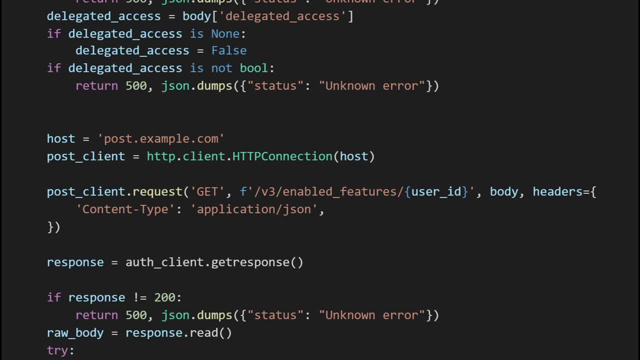 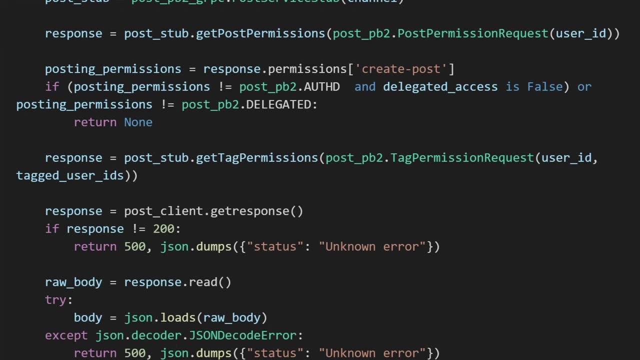 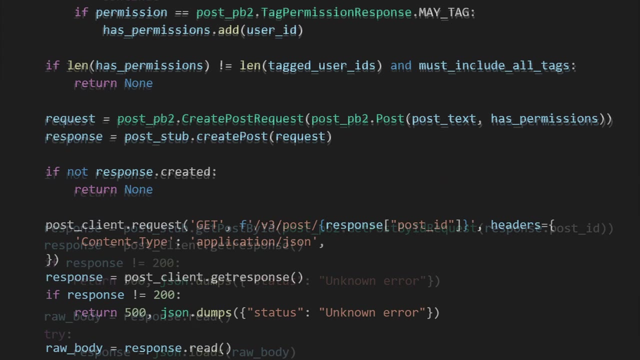 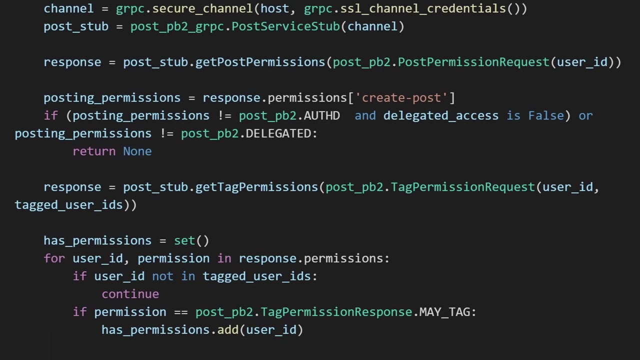 Now we just need to create the post service gRPC stub, replace this HTTP client with a gRPC stub and convert all the rest API calls to gRPC ones. With this done, we now use gRPC And I can actually read the code now. so that's. 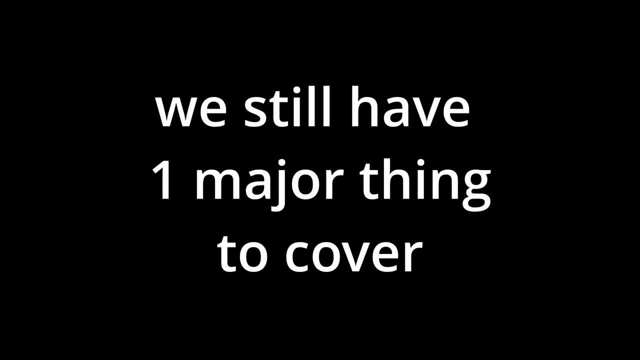 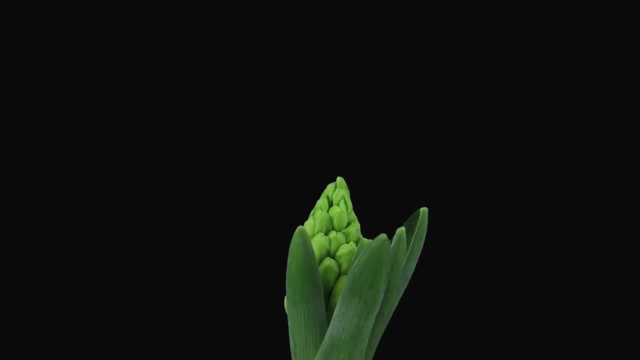 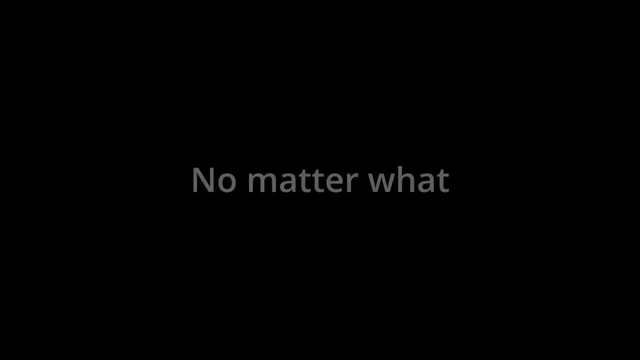 quite an improvement, But we still have one major thing to cover: How do we modify the API? After all, change is the only constant in software development, No matter what. you can break down API modifications to three things: Adding functionality, removing functionality or modifying functionality. Adding- 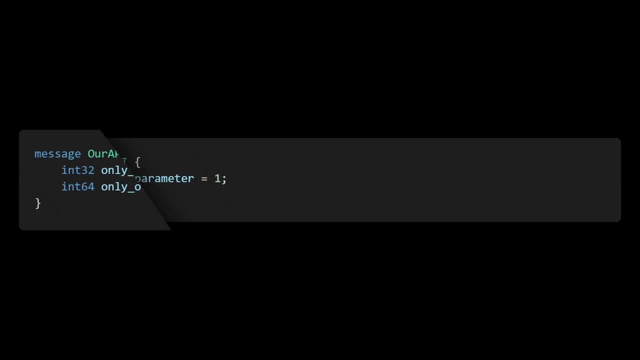 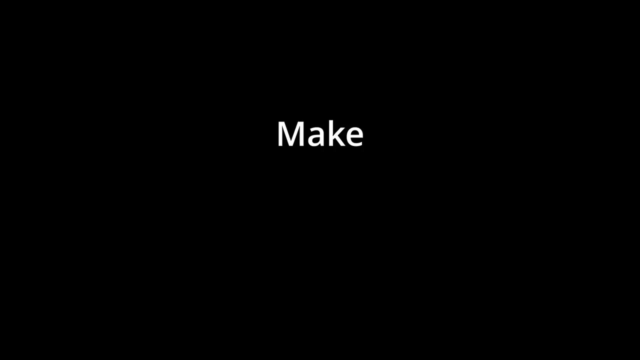 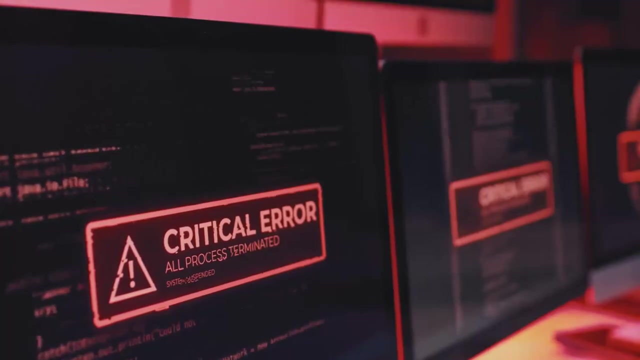 functionality is the easiest: Just add a field to the corresponding protobuf or add a new function to the service definition. But make sure that the API keeps working even if a client calls without setting the field. Otherwise non-migrated clients are going to break. 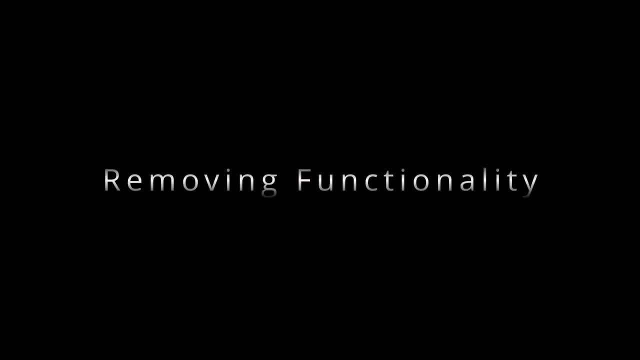 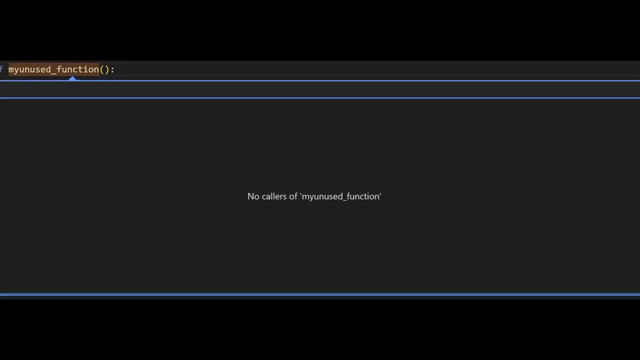 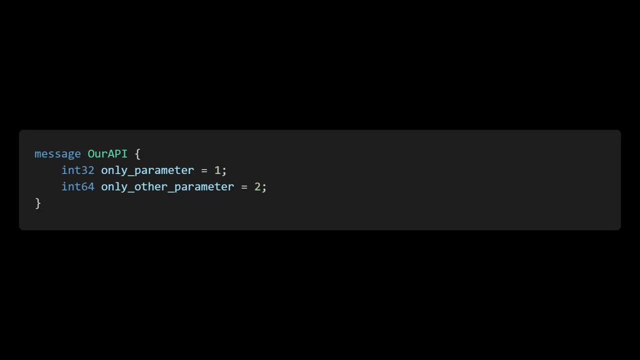 Removing functionality is slightly more difficult. First you need to make sure no clients are using the field or function you have created. If the API is widely used, that's a lot of work. But once you've migrated everything, you can safely delete the field or function. Modifying functionality becomes quite difficult.